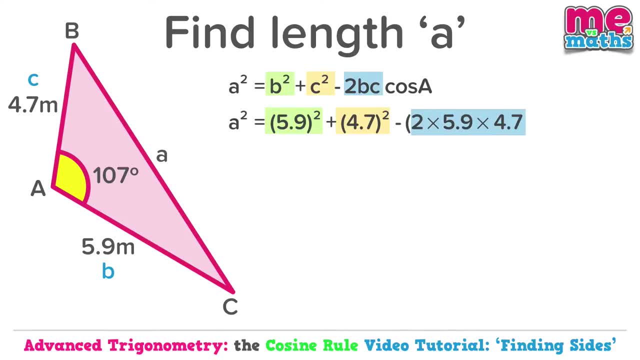 Minus. Open a bracket 2. times 5.9, times 4.7.. Then this part is multiplied by cos of angle A. So notice I'm still within that bracket. multiply by cos 107 and close that bracket off. Now, if need be, just pause the video. 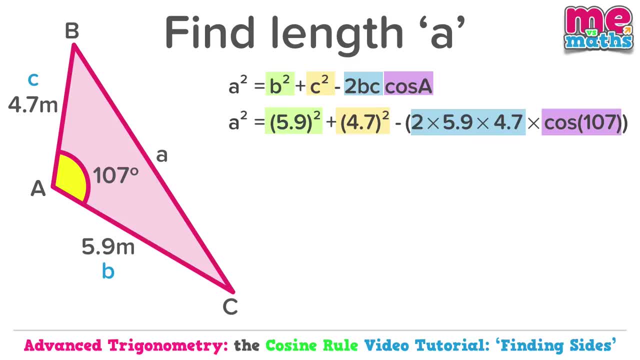 for a moment there and look over those first two lines, Check you're happy with how those different values match up. Hopefully the cos will help you to see which parts are which At this point, believe it or not, we're actually nearly finished. We can now enter everything on the right hand side. 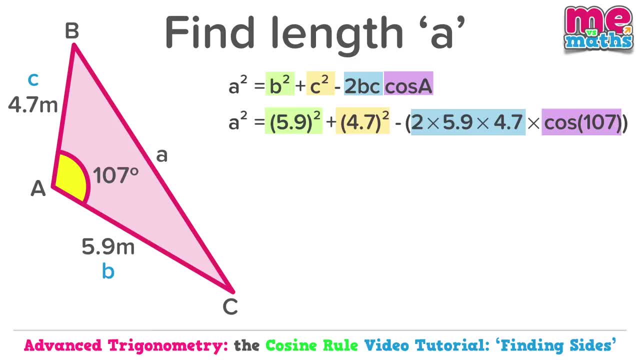 into a calculator, but- and I'll stress this again- you must do so very carefully. Make sure brackets are everywhere they should be and that you're not missing any of those symbols out. Okay, if you and I have both done that correctly, we should get 73.. 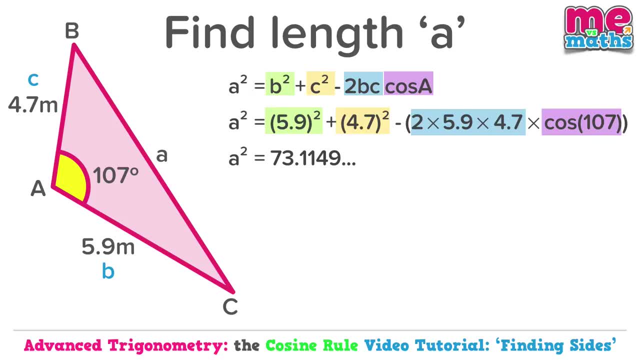 1149, and that's the value of A squared. So to actually find A, we need to square root this answer, Which, rounded off, should give 8.6 meters. As you can see, then, it can actually be quite quick to do, but you must be so careful with every small detail of your calculations or it will go wrong. 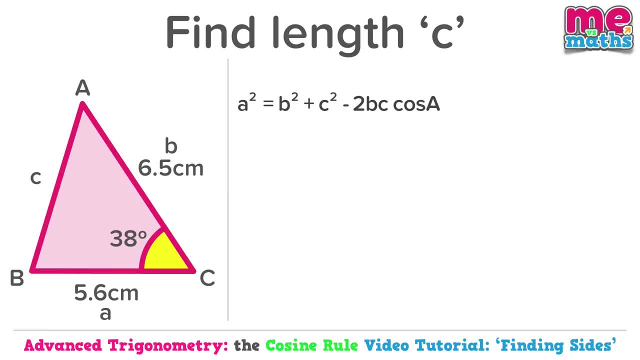 Let's look at one more question where we're being asked to do a question on the right hand side to find C. Now, questions like this have a tendency to cause complete havoc, in my experience, as it can be quite difficult to switch the letters around in the cosine rule. but let's have a go. 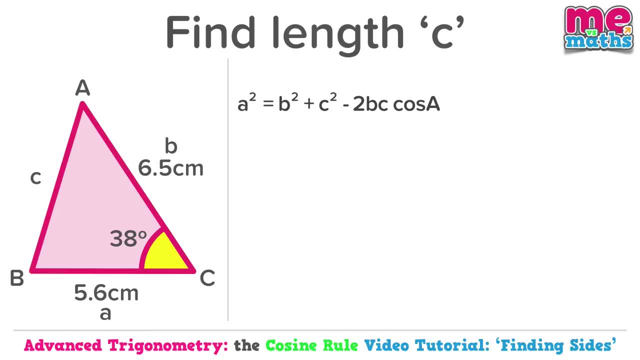 anyway and see how it's done. The important bit is the angle, As it's angle C that's marked in our triangle and angle A that appears in the cosine rule. we need to swap all our A's with C's and all our C's with A's. We can leave the B's exactly where they are. Let's look at the result. 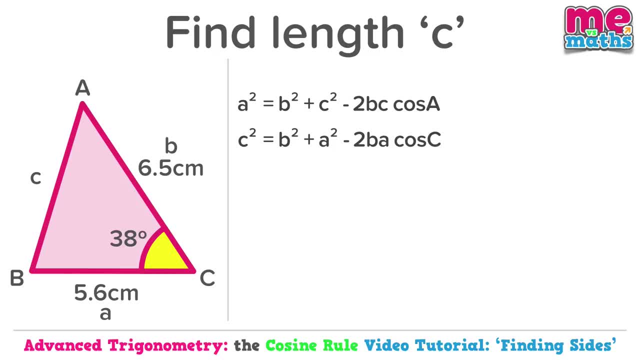 We said we'd swap the C's and the A's. so A squared became C squared. B squared stayed exactly as it was. C squared was switched to A squared. 2BC became 2BA And cos of angle A became cos of angle C. Right, that's definitely the most difficult part. Now we're able to just. 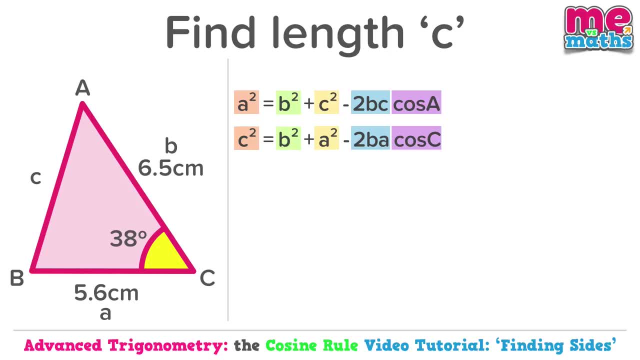 substitute our values in, as in the previous example. So C squared equals 6.5 squared plus 5.6 squared, The B 6.5, the A 5.6.. Don't forget to open that bracket. 2 times 6.5, times 5.6, das by cos thirty eight. 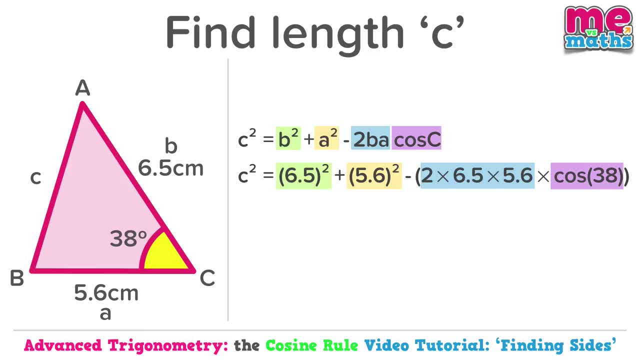 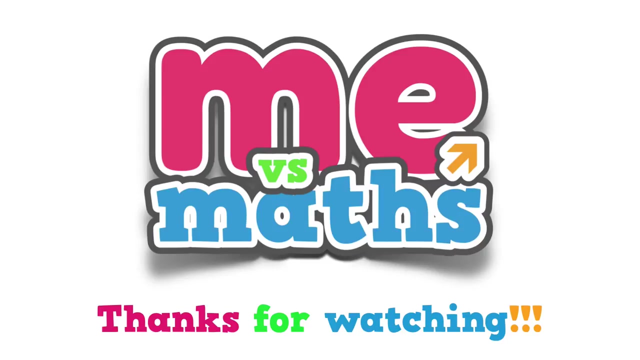 then don't forget to close those brackets off properly. So C squared is equal to 16.2428. let's square root that and find that C to one decimal place is 4.06.. Right, we're all done here on this topic. thanks for watching, as always. 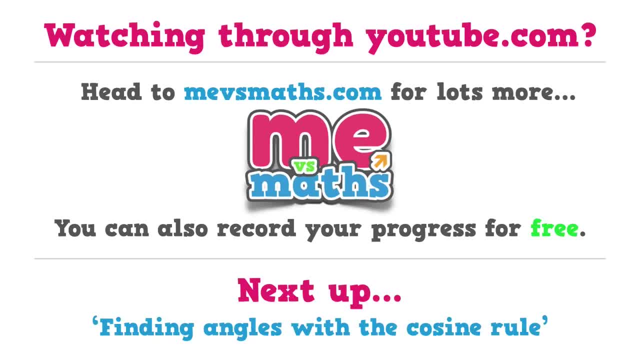 In our next tutorial, we'll continue to look at the cosine rule and this time use it to find angles rather than sides. Don't forget, you can find plenty more resources on the website, and if you have any queries about any part of this tutorial, then please just let me know in the comments section. 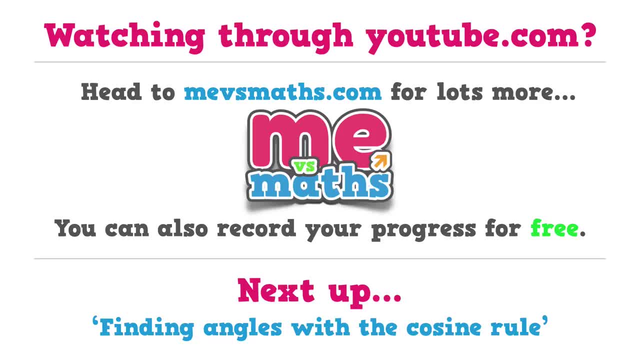 Thanks again and bye for now. Subtitles by the Amaraorg community.